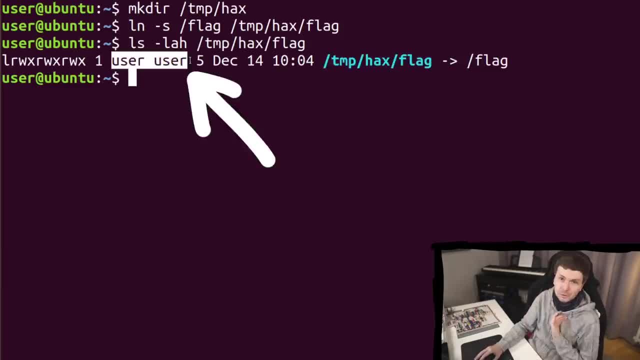 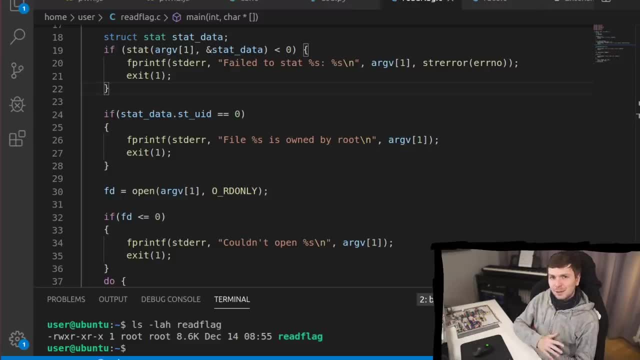 a symlink And the symlink now points to the flag and the symlink is owned by the user. So let's try it. Ah, doesn't work, So let's do the raise condition. Like I said in the beginning, I want to show you a raise condition problem. So we have a raise condition here. So when it calls: 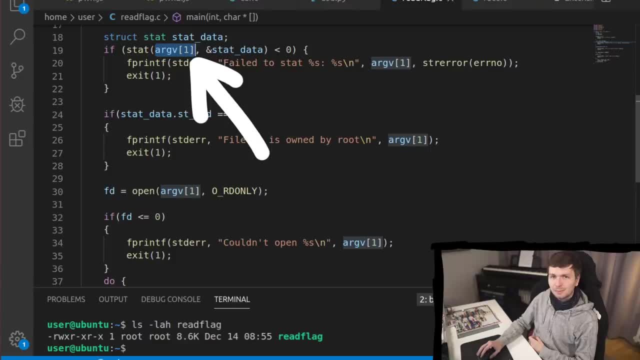 start to get the file information, it uses the file path And when the check succeeds it uses the file path down here in the open to open that file. So basically we want to win here a raise where when we call start for the first time on that file, it's just a save. 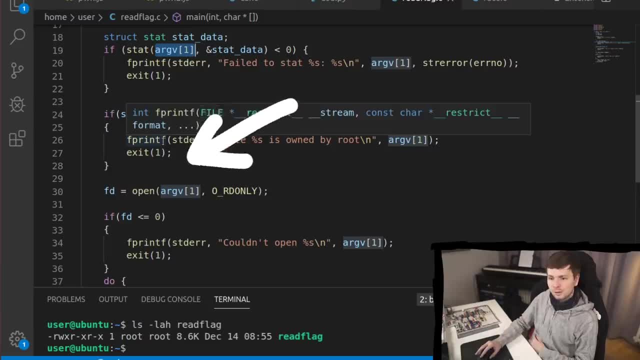 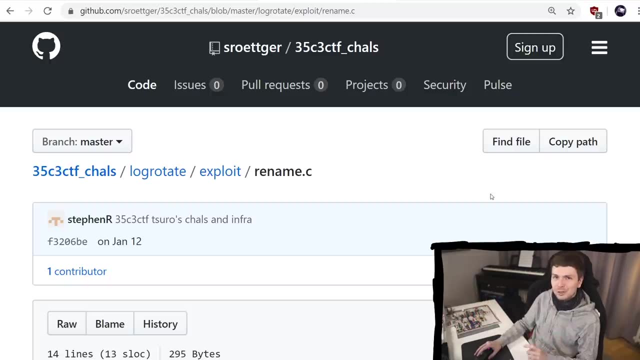 file, But when the program then continues to execute, we switch it out, And when it then reaches the open, it will then actually open the file that it shouldn't have opened. There's a very useful raise condition snippet that I learned about at the 35c3 CTF. 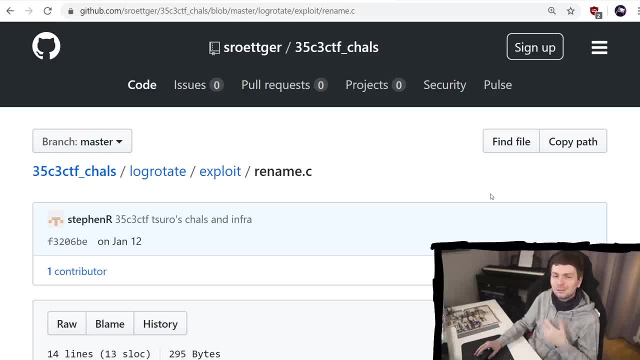 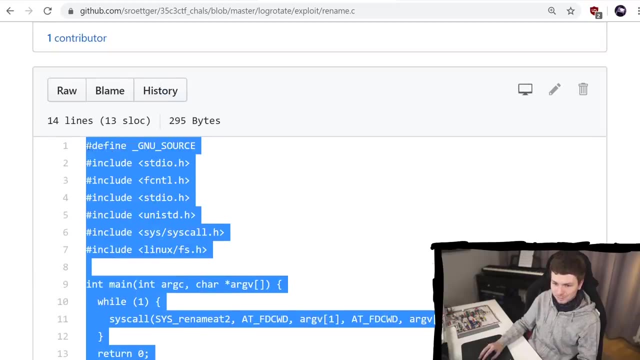 from the challenge lock rotate. I didn't solve that but after CTF- talking with might have been Niklas B at the time- he told me about that. there's basically a syscall to swap two files And that is really, really useful. So here's the code. let's copy that and I explain in a moment. 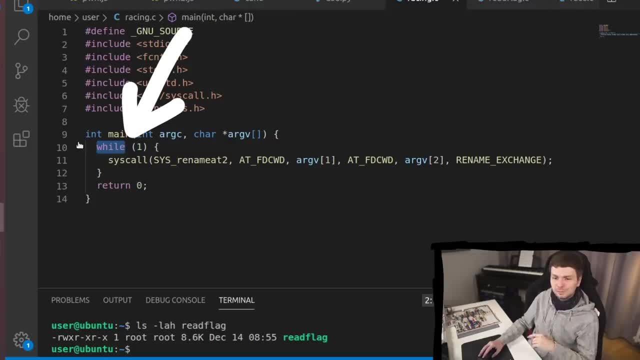 So here we have a while loop Just calls a single syscall And the syscall that we are calling is called rename, add to. It takes some parameters, but the most important ones are this one and this one. These are two file paths And we use the option rename exchange. So basically that's a rename. 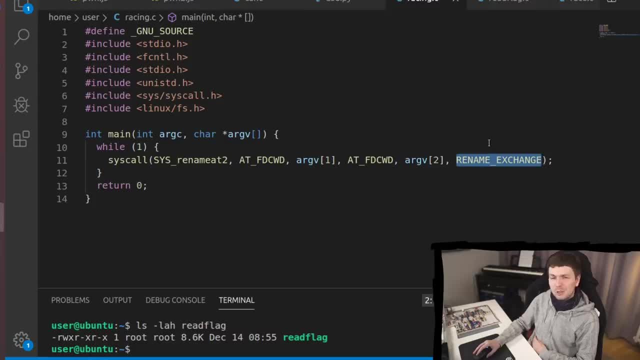 system call to rename files And with this option, rename exchange, you can actually switch, exchange the names of these two files. So basically, this syscall with this option is just a raise condition syscall. It's a really awesome Linux feature, So let's compile it So in this. 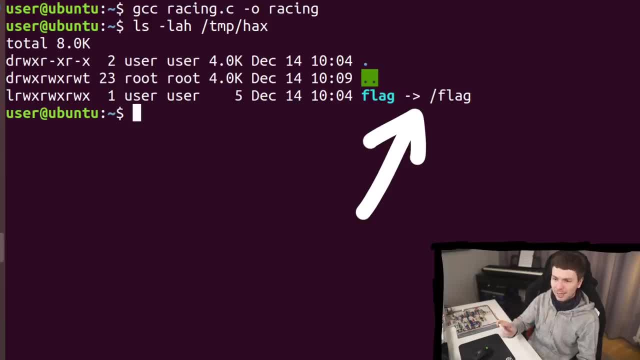 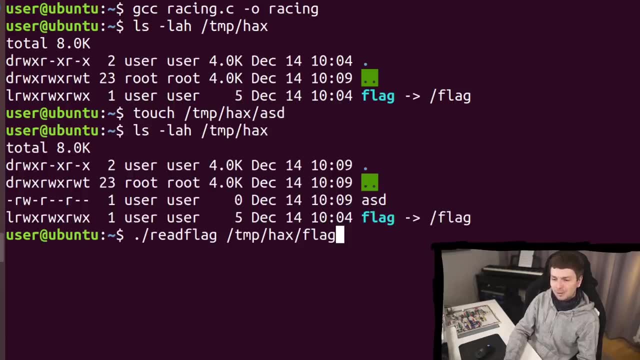 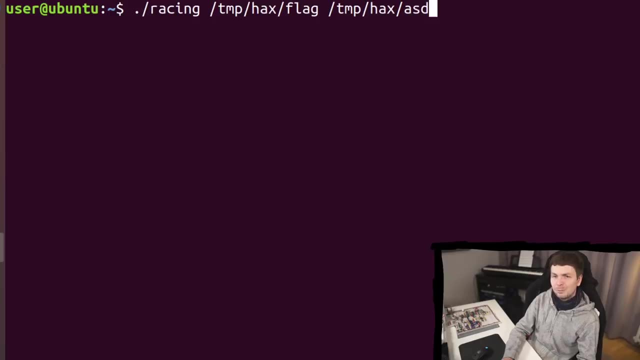 folder tmp-hacks, we already have this symlink to the flag, so we just need another file. So, now that we have an asd file and we have the symlink to flag, Now remember, when I try to simply read the flag file, we say it's owned by root. But let's launch our small raising program. 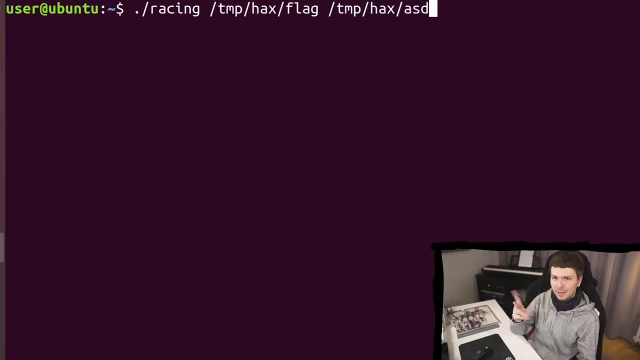 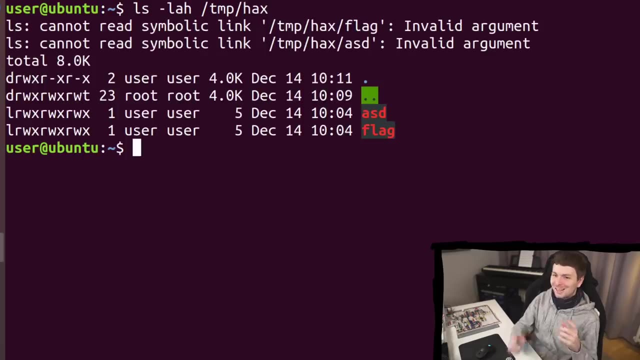 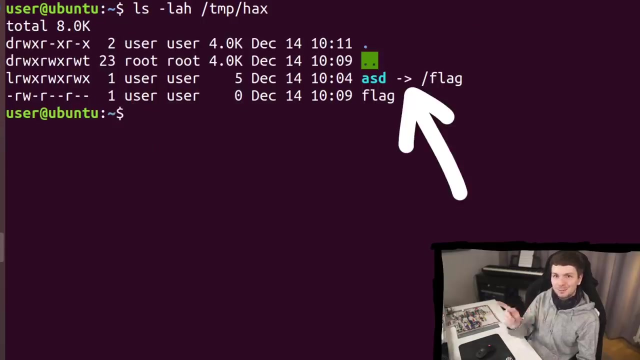 We specify in the arguments the two files that we want to constantly exchange and switch with each other. So now it should be executing. So let's check out the folder. Okay, now this is switching so fast around that ls here even threw some errors. Ah, look here. this time asd was pointing to the flag and the flag was just a valid. 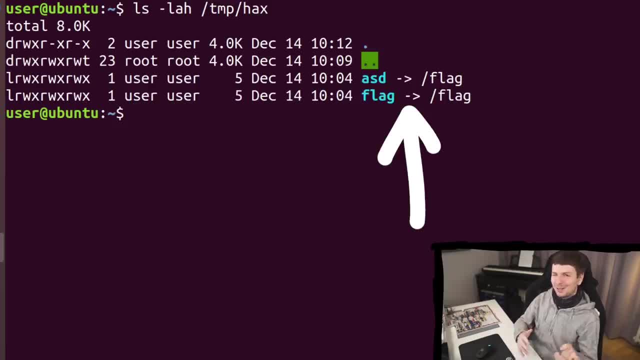 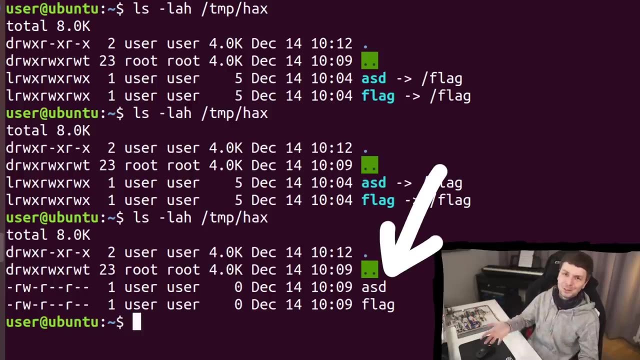 file. Now, ls was kinda so slow that the exchange happened so fast that it thought that both files are a symlink to flag. Basically, we just raised ls And here we raised like the inverse. Now both files are pointing to flag. Anyway, now let's try read: flag Owned by root. It didn't work. 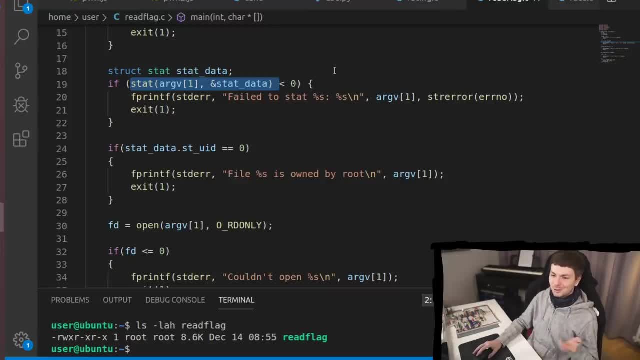 There we go. We won the race. That's awesome, right? So basically, during the first start, the flag file was just the regular file, and then, while it was executing here, a bit more code. our raising program exchanged the files again, and when it then opened it, it actually opened the real root owned file. 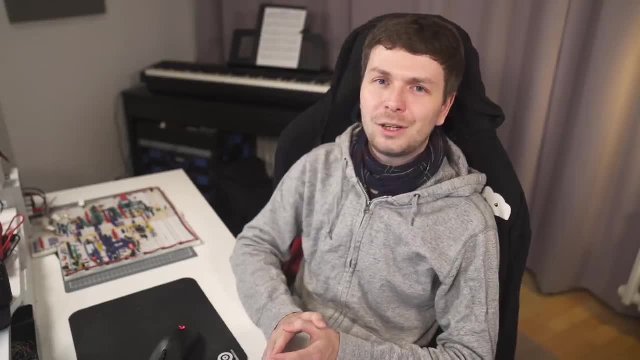 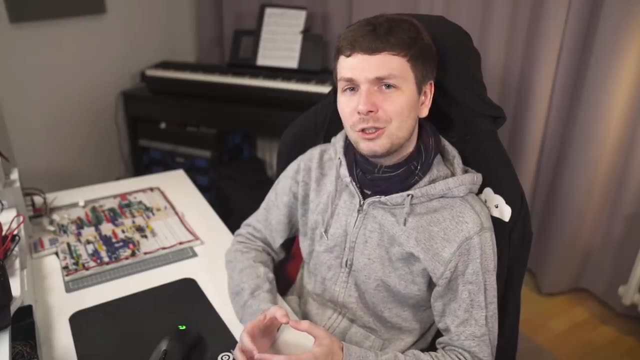 Race conditions are pretty fun. It's a very typical bug pattern that you can find, Especially always when you are dealing paths. So when you are auditing code or playctf challenges, always pay attention to if this program that you are targeting is handling file paths And check if. 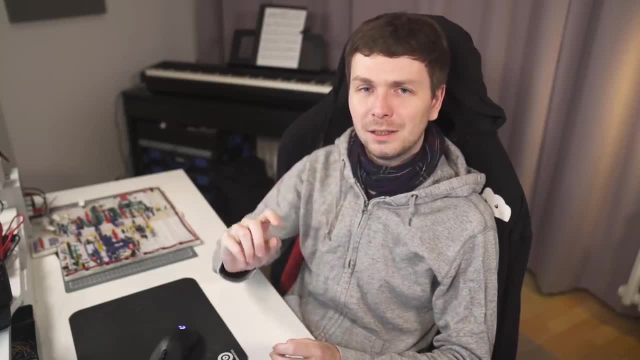 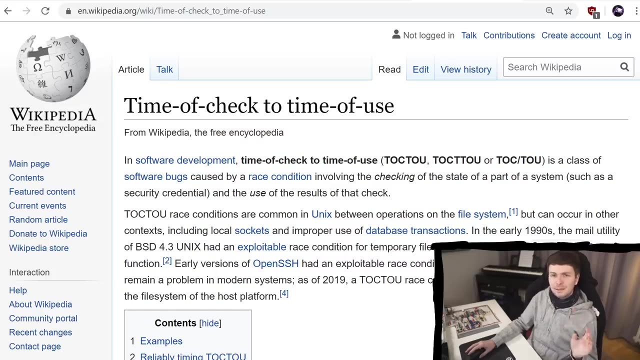 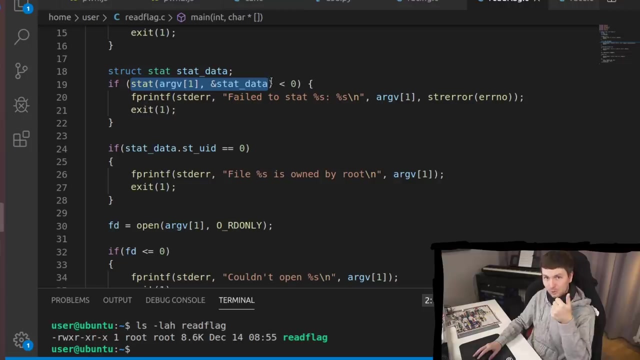 it always trusts the path and if you have some ability to race between the first time it uses the path and the second time it uses the path. Just for completeness sake, this issue is often also referred to as TOC2.. Time of check- time of use. During the time we checked the file, it was ok. 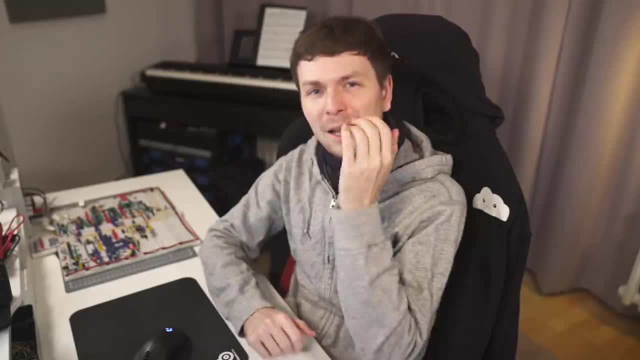 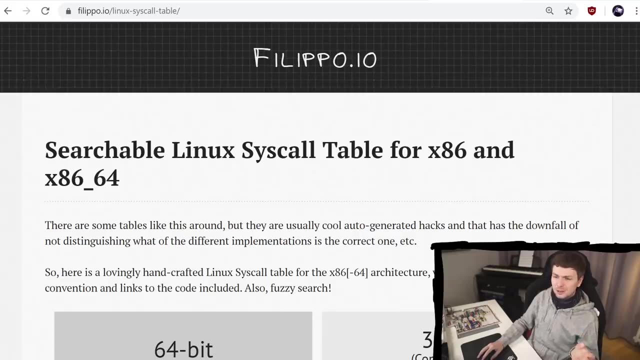 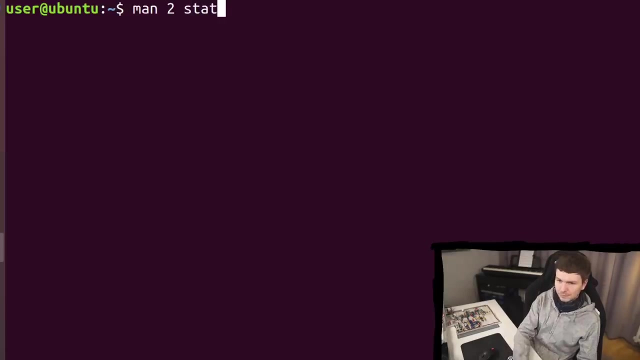 During the time we used it. it was then bad, But how can you avoid this? now? This seems like a problem that is almost like unavoidable right. STAT is essentially a syscall. So let's look at the syscalls. So on 64bit, on linux, the STAT syscall is syscall number 4.. And when we look, 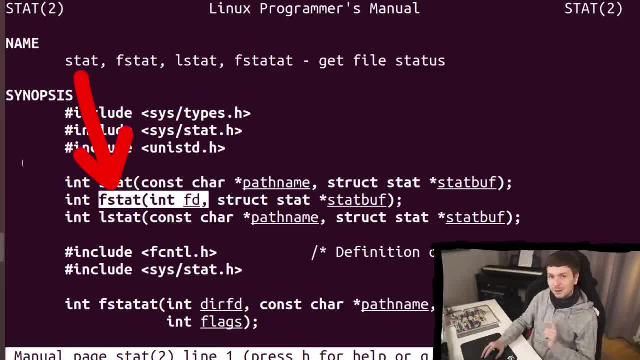 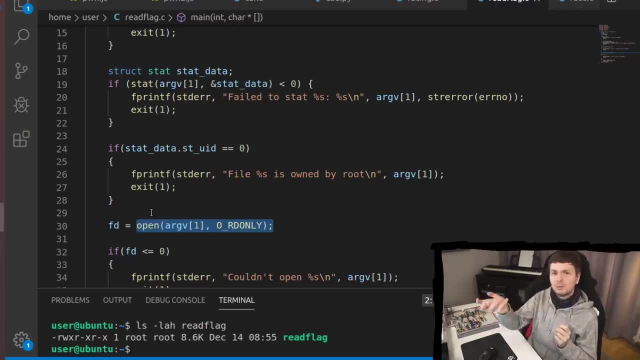 at the main page we see that STAT takes a path name, But there also exists fstat, And fstat is another syscall, The syscall with number 5. And that syscall takes a file descriptor instead. A file descriptor is a handle that points to a specific file And, for example, the open syscall. 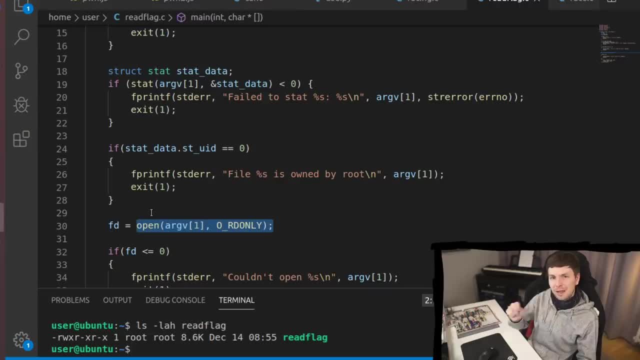 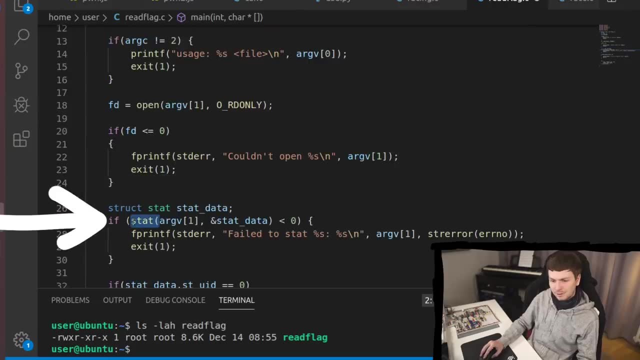 returns a handle to that file. Which means, if we wanna use fstat we need this file descriptor. So we have to move the open further up before the stat And then we refactor fstat to take the file descriptor instead. You can already see that now we only use the file path once. 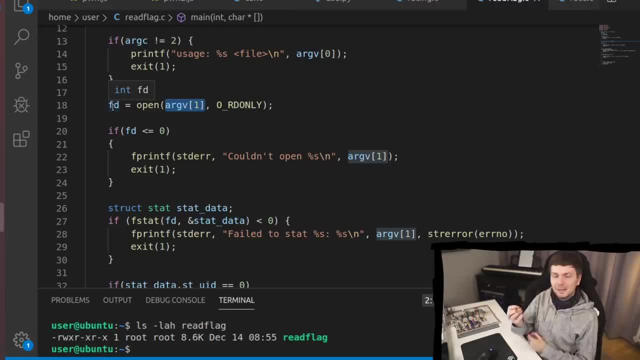 The file path is used to open this file and get a handle, And this handle just points to that one file. There is no way to exchange this anymore. Unlike file paths, a file descriptor, this number is a handle for a file that is deeply rooted. 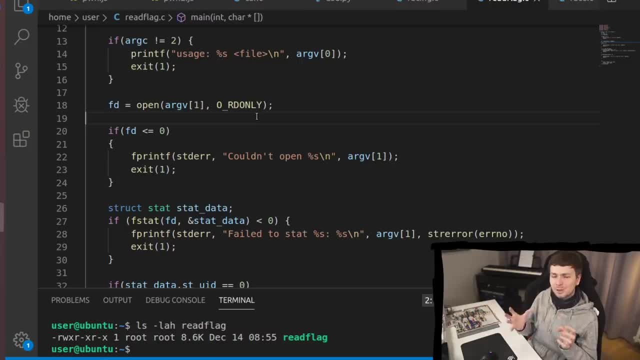 inside of the linux or unix operating system At this moment in time there is basically no concept of a path anymore. This is now a thing that just represents that one file And you can't switch that anymore. That file descriptor just points to that file. 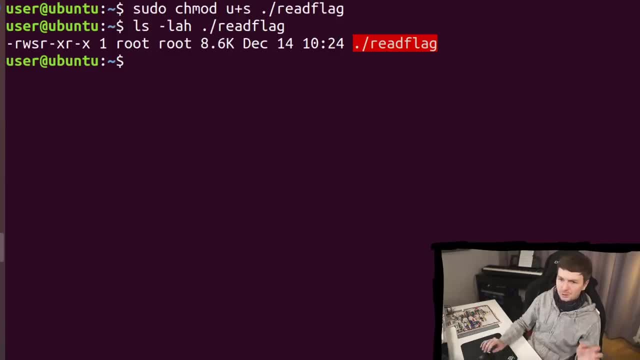 So let's compile this flag and let's try our race again, And also making it set UID binary again, so we have the same basic setup. So here we execute first our race condition program again, And now let's try to execute this. Okay, so there was no error. 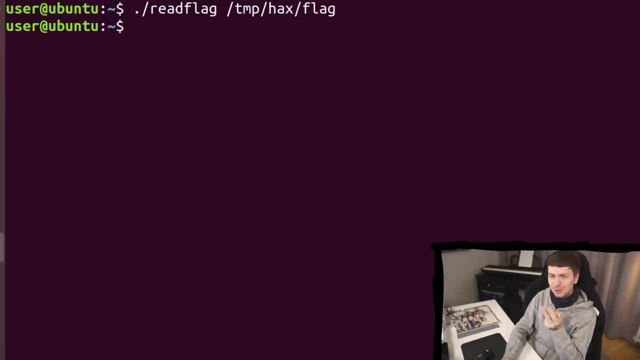 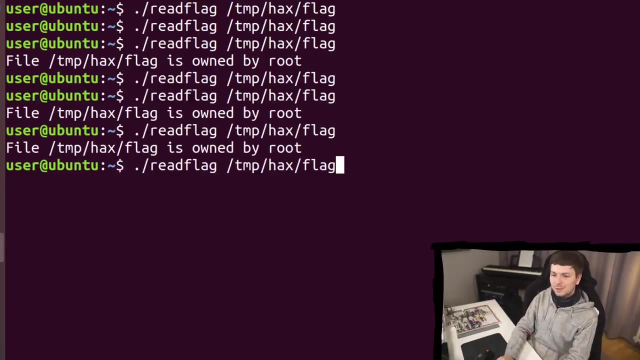 Which means now, probably because of the switching, we pointed to the empty valid normal file, Normal file. ah, there we go Now. this time it was again the actual root file And when it now tried to read it we get the error. But as you can see, 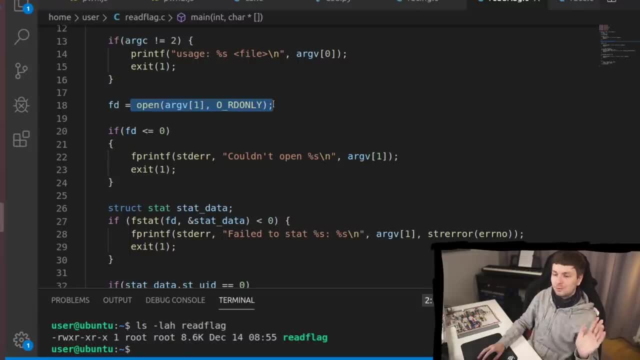 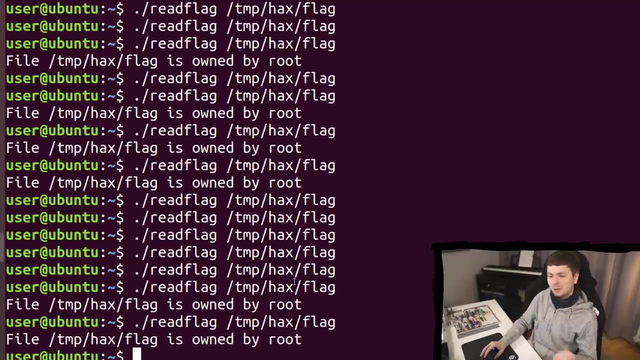 no chance for race condition anymore. Now it only depends on which file is there at the moment when we open it. It was either the regular user file, which is empty and doesn't print anything, Or it is the root own flag file, And whichever of the two is opened during the race will either print the empty file. 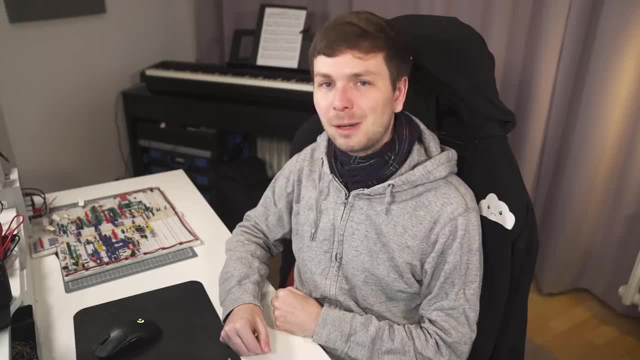 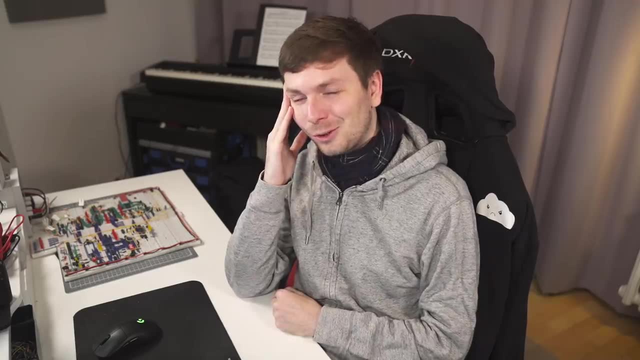 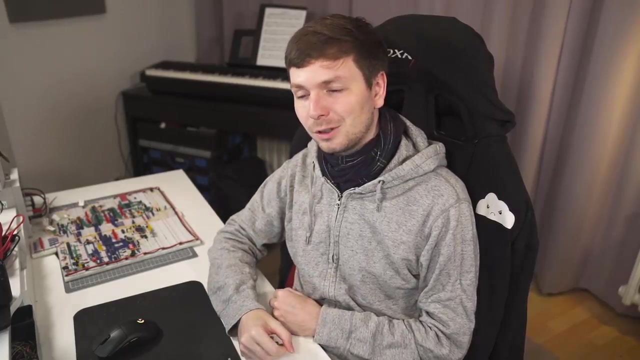 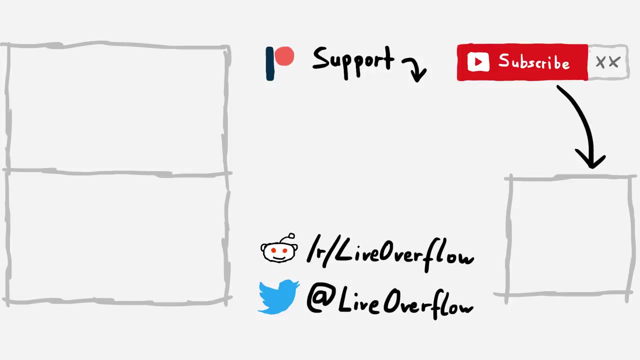 or cause then the error. So we have prevented the race condition. Crap, I'm sick. That's not how I planned these 24 hexember daily videos to go, So I was out for a couple of days and couldn't prepare more videos. I guess now it's even more likely that I won't be able to deliver all 24 videos.